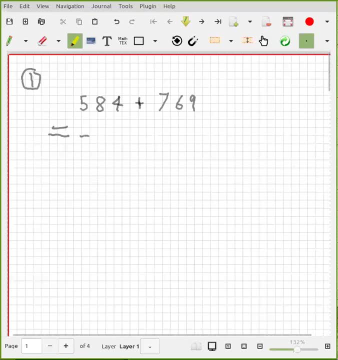 Let's do that and you'll have to forgive my my problematic number writing. Okay, Now, if you notice this 8, this 28 10s here is only two 10s away from 300.. So let's take two 10s from this 60 here. 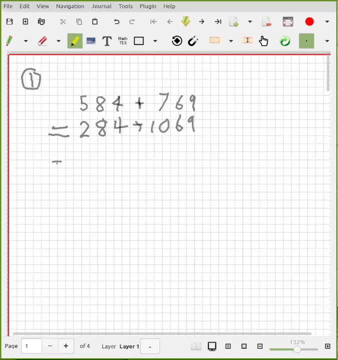 Let's take 20 from this 60 and add it here and we'll get 304.. Because we added the two here and we'll end up with Because we took away two here and we added them in here. Okay. 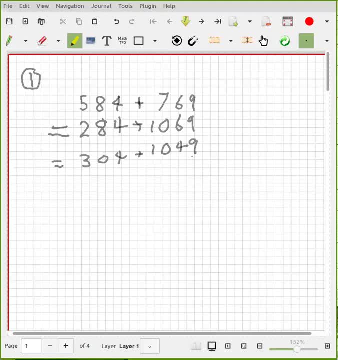 Now the last one: this 4 and 9, if we This, 49 here is only one away from 50. So if we take one away here, we'll have 303.. 303 plus 1050.. Now I can just 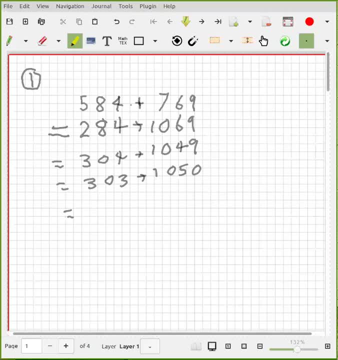 There's no caring involved in this sum, So I've transformed the sum, with some complexity, into a sum that's fairly simple. We can just write 1, 3,, 5, 3.. Okay, Okay, So this involves a little bit of having to sort of do a little bit of thinking. 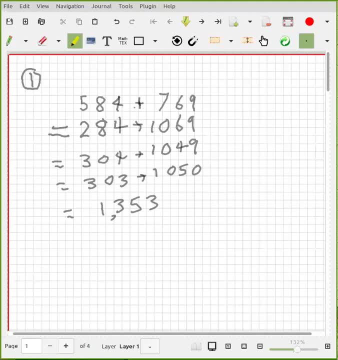 The standard algorithm avoids thinking, But the problem is that when you're designing computer algorithms, that's what you need to do: You need to think about new ways to solve problems. Okay, So let's go on and try one with subtraction. 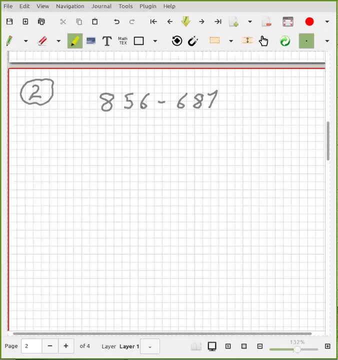 Now the principle to use here is: if I add or subtract the same amount to the sum, the difference stays the same. So let's do that. We can notice that here we can take this: There's 6 here and 8 here. 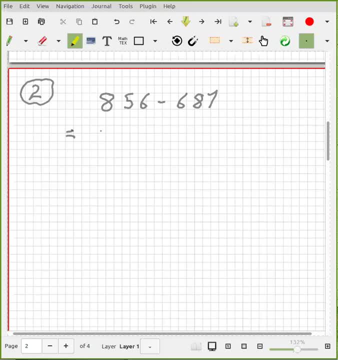 We can take the 6 away from the 8 and both We can get. This is going to be 256 because we're taking 600 away from both, Okay, Okay, Now this 8 is too large for the 5.. 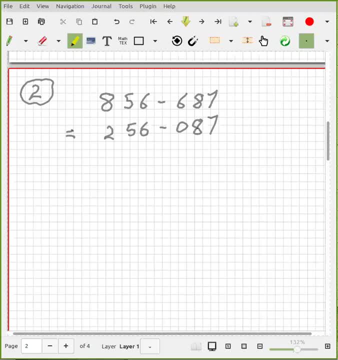 So what we want to do is we want to raise this up, So we want to get rid of this 8 somehow, And the way to do it is to add 2 here at the expense of adding 2 here. So let's do that. 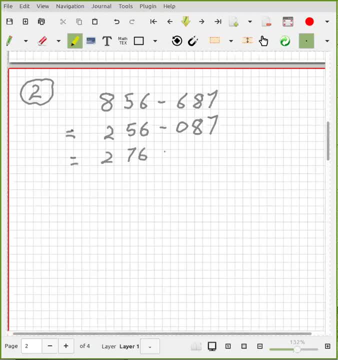 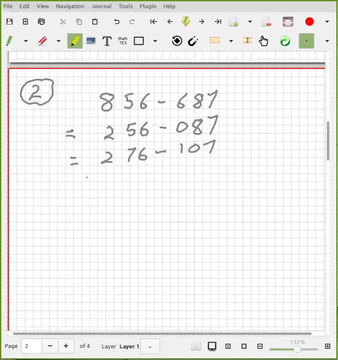 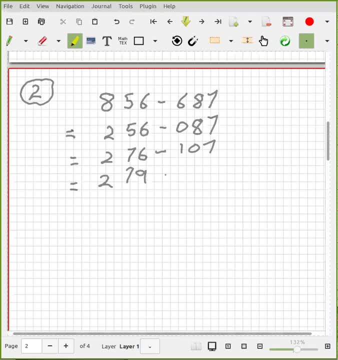 So we end up 279 minus We've added 3.. 1, 1, 0.. So now 2 minus 1 is 1.. 7 minus 1 is 6.. And 9 minus 0 is 9.. 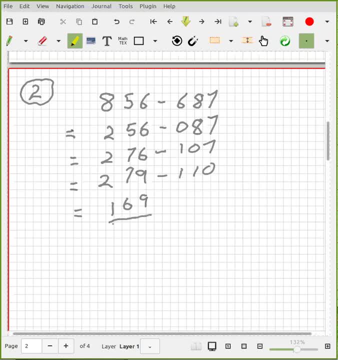 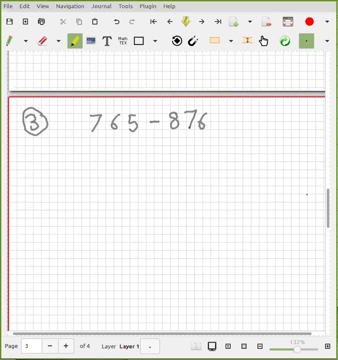 And that is indeed the right answer- 169.. So So Here the idea was, we used a different principle. We used the same idea of sort of applying a mathematical insight and then looking for patterns in the numbers- Well, this was subtraction. with this number larger than this, How would it work? How would the same idea work with this number in which the 765 is less than the 876?? 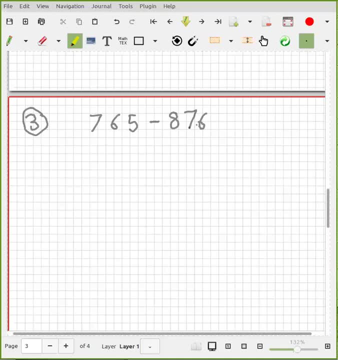 Well, if we could drive this one down to zero, we would have the answer over here. Well, right away you can see if I take, because it's a difference. So if I take, I can take away something. I can take away something from both sides and it won't change the value. 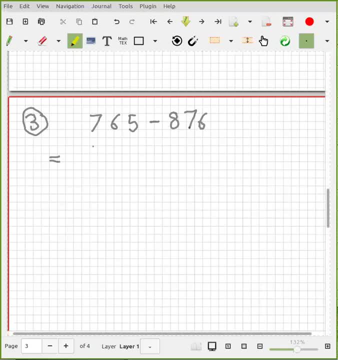 So I can take away 700 here and 700 here, So I take away the 700, and I end up with just 65, because that goes to zero And we have got 176.. Now, again, this number is less than the 7, so we can do the same thing and subtract 6 from both sides. 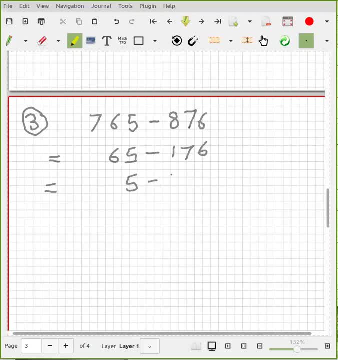 So we're going to end up with just 5 minus 116.. And we can take 5 away from both sides there and we're going to get 0 minus 111. So the answer is negative 111, which is indeed the answer. 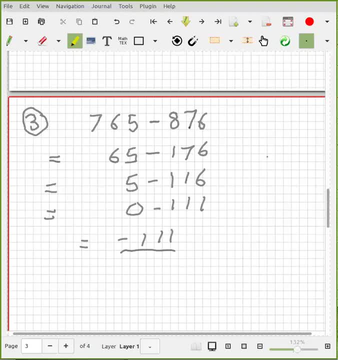 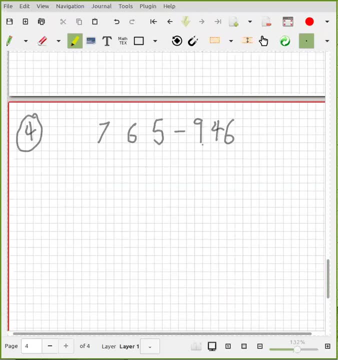 Okay, so this was all. of these digits were larger than this one. What happens if you have a mixed thing, which here see, the 7 is less than 9, but the 6 is larger than the 4. And again, the 5 is smaller than the 4.. 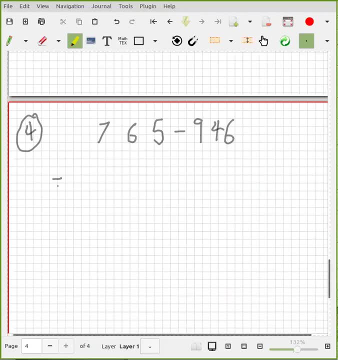 Well, We can do the same thing. We can just see if the same thing works of subtracting the 7 from both sides to get 65 minus 246. But here what we can do is we can do something a little different, because instead of pushing this down to zero, 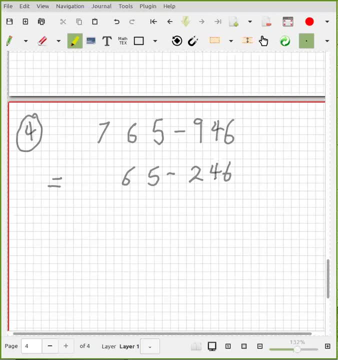 because if we did that that would go less. what we can do is we're going to add 4 to both sides to push this up. So if we add 4 here, that's going to give me 105 minus 286.. 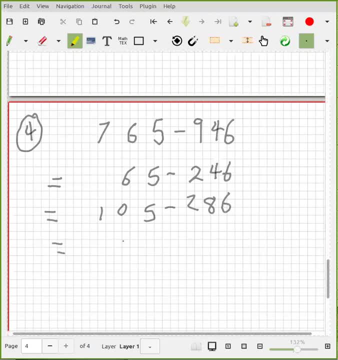 Well, we can push this 1 down again, So we're going to end up with just 005 minus 186.. And then we can push this 5 down to 0, which gives us 0 minus 1, 3, 6.. 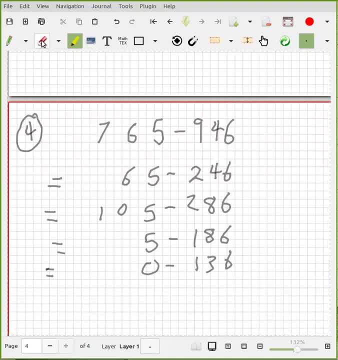 Oh, that was a mistake Here. Why did I? This is a 5.. So when you push this down, we're going to take 5 from the 1's place. This is going to be 0 minus 1, 8, 1.. 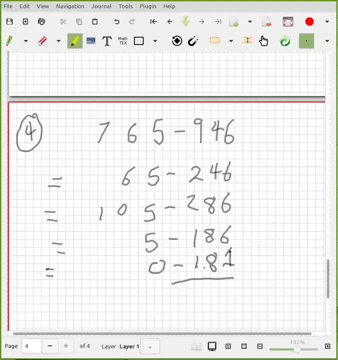 And that is, Indeed, the right answer. OK, so this is how you can use insight to think that this kind of doing arithmetic is actually a little bit more enjoyable than the traditional means, which is: you be a machine, you be a computing agent. 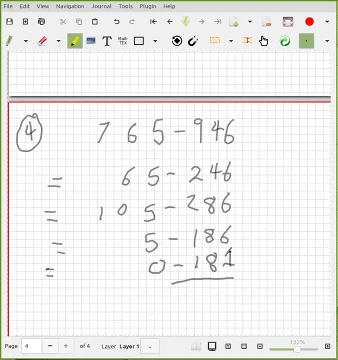 So I think that's it for this topic.